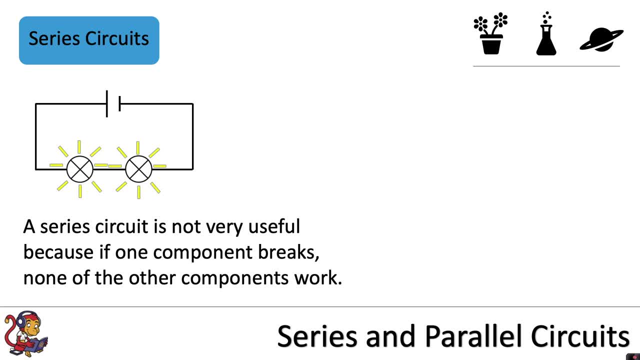 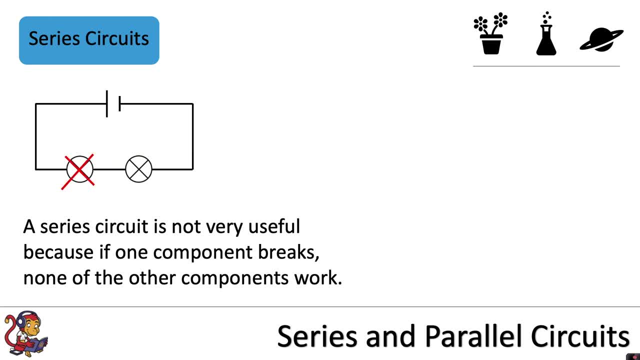 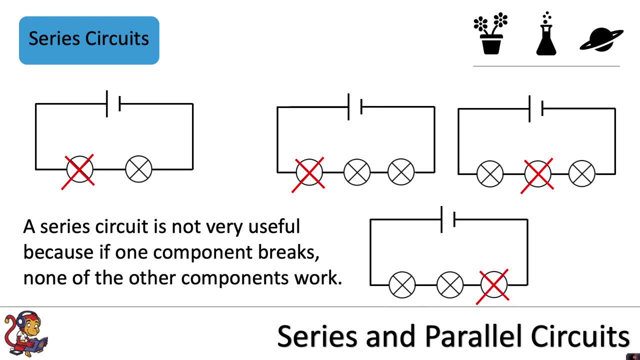 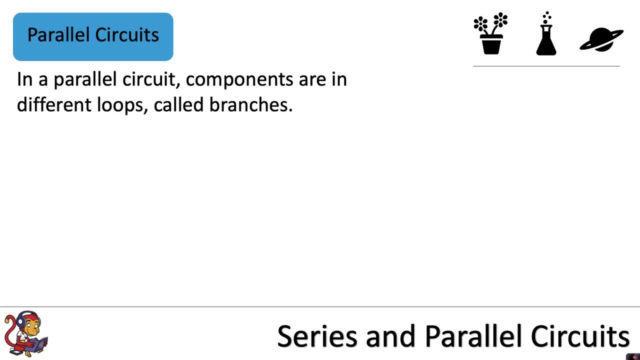 or the third lamp, Wherever it is, it will mean that the circuit is now broken and all of the components will not work. In a parallel circuit, components are in different loops, which we call branches. So here, when we're adding a second lamp in rather than putting it in the same loop, we add 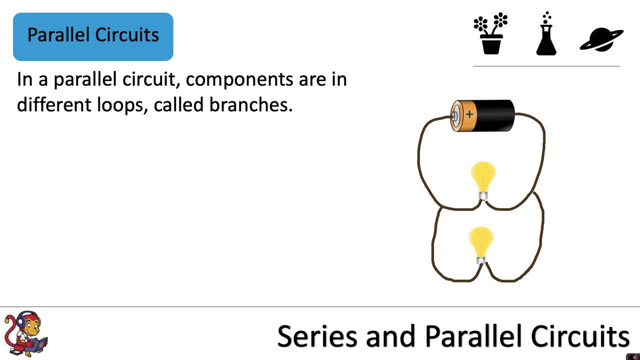 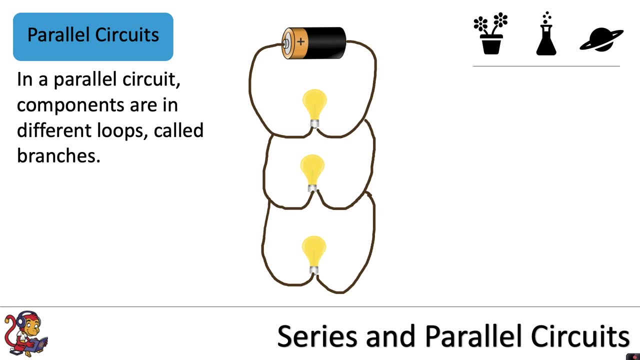 a second loop of wire and put the component in its own loop of wire. The circuit diagram would look like this and you can see the parallel lines which lead us to call them parallel circuits. Or if we were to have three lamps in a parallel circuit, it would look something like this: A parallel- 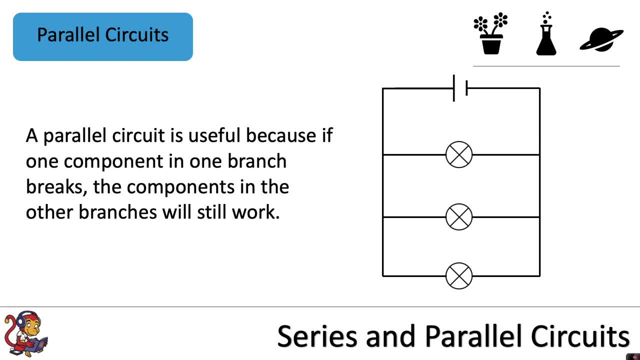 circuit is used to connect two lamps in a parallel circuit. If we were to connect two lamps in a parallel circuit, it would look something like this: This will also show that if the last lamp in the second branch breaks its first lamp and the second lamp breaks its second lamp, This is useful, because if one 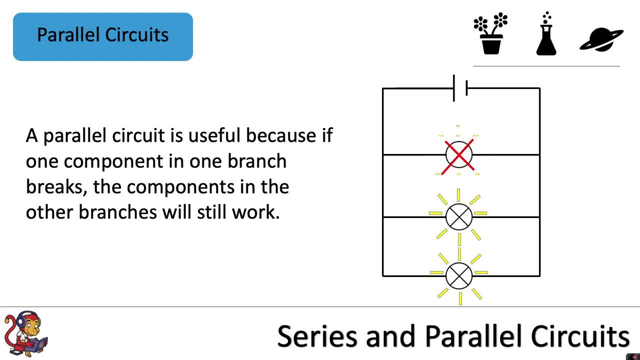 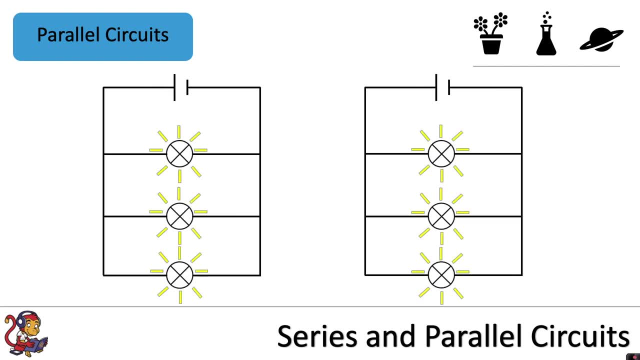 component in one branch breaks, the components in the other branches will still work. For example, if these three lamps were shining brightly, if the lamp in the first branch were to break, the lamps in the other two branches would still work. Similarly, if the lamp in the second branch broke, 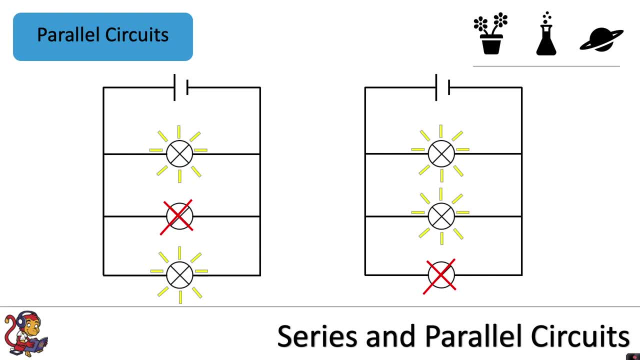 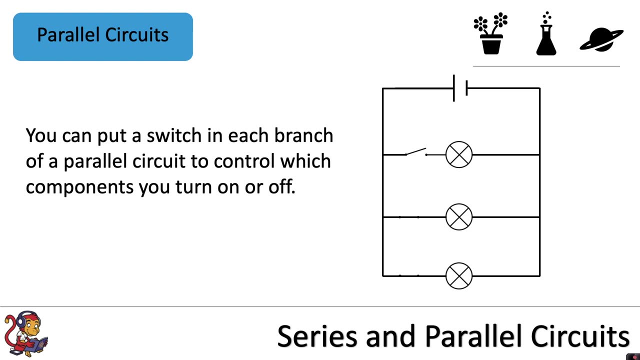 branch broke, the lamps in the first and second branches would still work. So these circuits are much more common because they're much more useful in comparison to the series circuit. You can put a switch in each branch of a parallel circuit to control which components you turn on or off For. 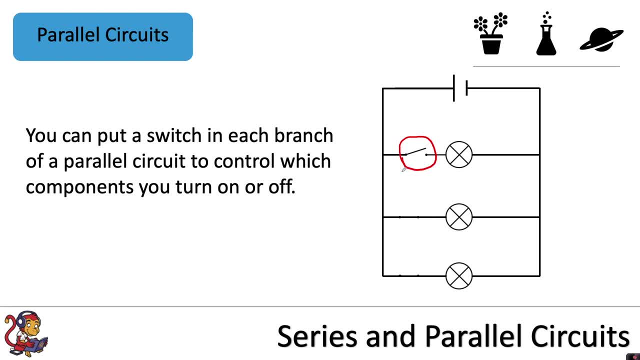 example, here we have an open switch in the first branch, a closed switch in the second and a closed switch in the third. So in the first branch we've got an incomplete circuit. so whilst this switch is open, the first lamp would not light up, but the other two would. So we are in control of which lamps are on and which. 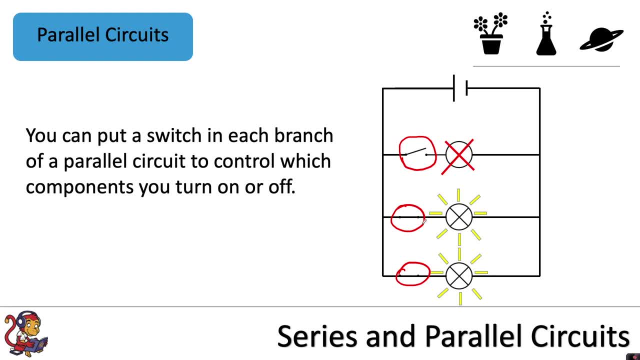 lamps are off just by putting these switches And, of course, if we wanted to turn this lamp off, we would open up this switch and if we wanted this lamp to shine again, we would close it. So we are in control of which lamps we turn on and off In a. 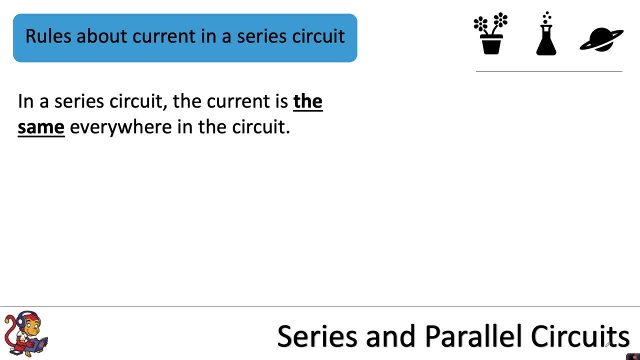 series circuit. the current is the same everywhere in the circuit. Remember, the ammeter is placed in series with the components in the same loop and the ammeter is what we use to measure current. So in this series circuit here we've got two lamps and I've just put three ammeters in to show that the 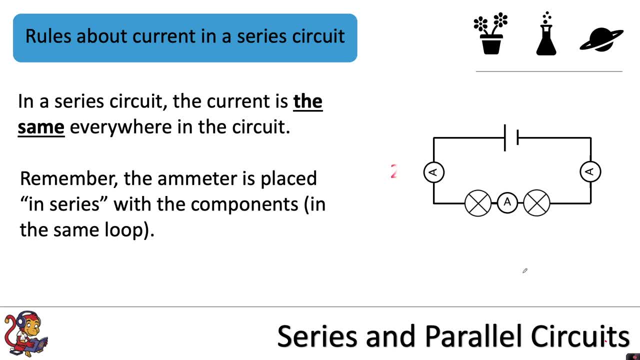 current is the same everywhere in the circuit. So if we were to measure two amps of current here, the rule says it's the same everywhere. so here we would also get two amps, and over here we would also get two amps In a different circuit. 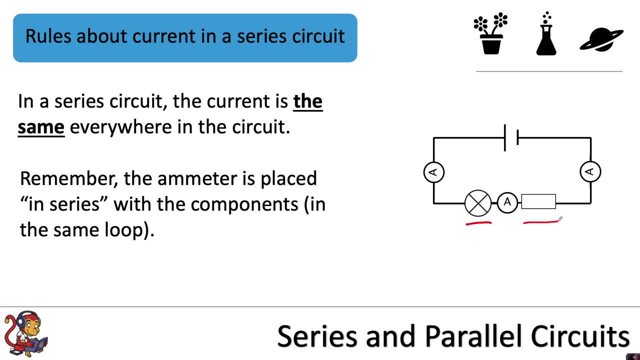 now. I've now got a lamp and a resistor in my series circuit, So the current may be different here, but the rule is still the same. The current is the same everywhere in the circuit. So, for example, if when we change our components, our current was now one amp over here, it would also be one amp over here and one 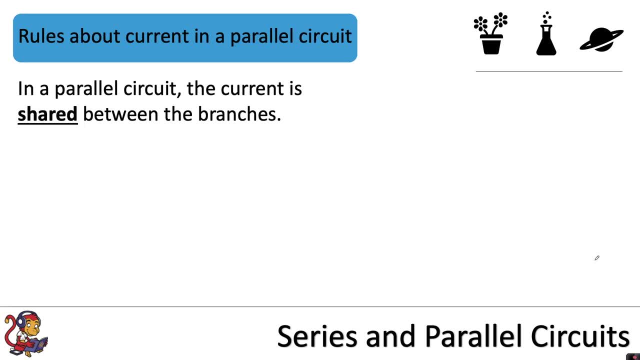 amp over. here. In a parallel circuit the current is shared between the branches. The ammeter at the top next to the cell will show the total current. The ammeter readings in each branch will add up to the total current. So if the total 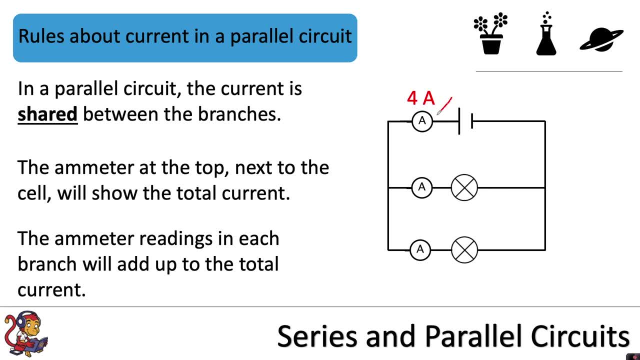 current was four amps, measured by this ammeter here next to the cell, then these two ammeters should both add up to four amps, and because we've got the same component, we'd expect the same current through each branch. So here we've got two amps through the first branch and two amps through the second branch. So 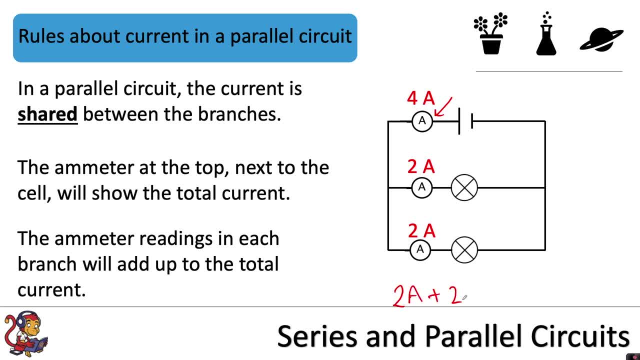 each branch. two amps plus two amps will equal the total current at the top of four amps In a different circuit. now we have one lamp in the first branch and a resistor in the second branch. Let's say that the total current was again four amps. The same rule applies in that the current is shared between the branches. 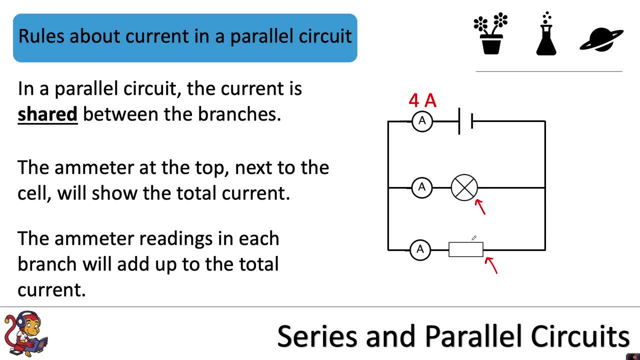 but this time, because it's two different components, the current is going to be shared unequally, So, for example, we may have three amps flowing through the first branch and only one amp flowing through the second branch. However, the rule is still the same: We will add up the current in each of the 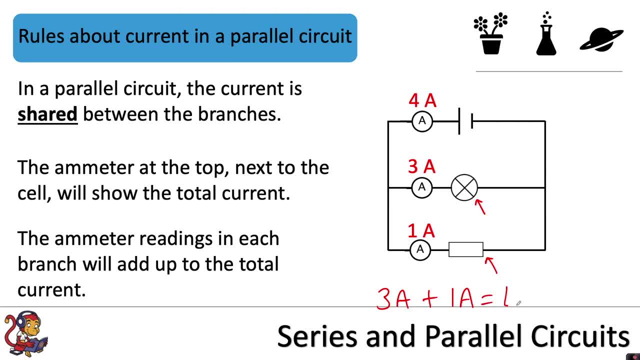 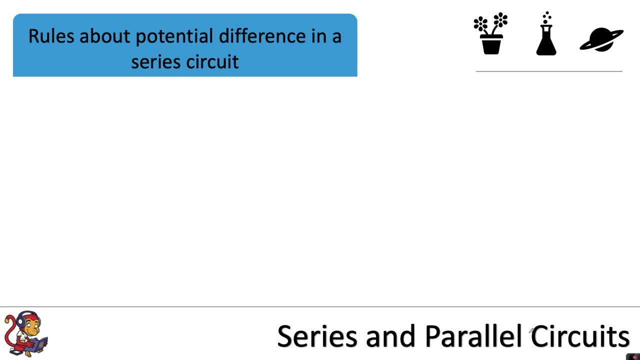 branches and that will equal our total current of four amps. Now we'll move on to rules about potential difference and first look at the series circuit. In a series circuit, the potential difference is shared between components. The potential difference of each component will add up to equal the potential difference of the. 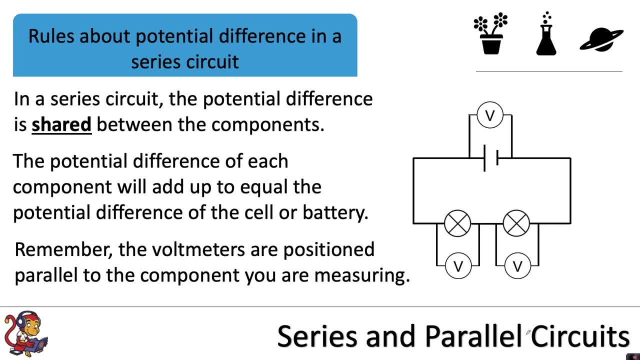 cell or the battery. Remember, the voltmeters are positioned parallel to the components you are measuring. So the voltmeters are what we use to measure potential difference, and what I mean by they're positioned parallel to is that we have to have these separate wires. 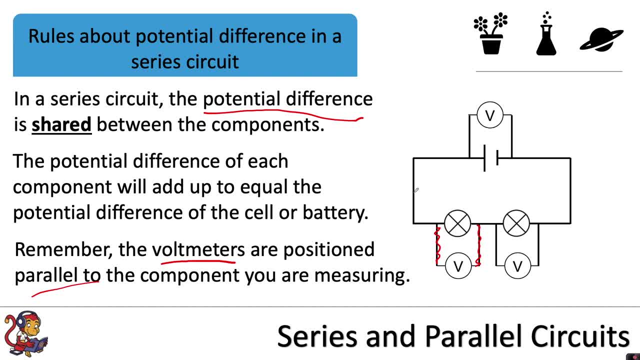 coming down to connect the voltmeter. We do not place a voltmeter in the same loop as everything else, Whether it's series or parallel. you have to connect the voltmeter with these two wires going down either side of the component. So our 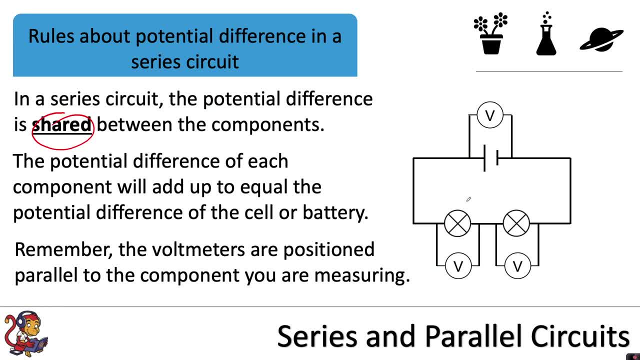 rule says the potential difference is shared between the components. So if our total potential difference provided by the cell was six volts and we've got two of the same components, two lamps, here, this will be shared equally. So three volts to the first and three volts to the second, and each of these will add up.